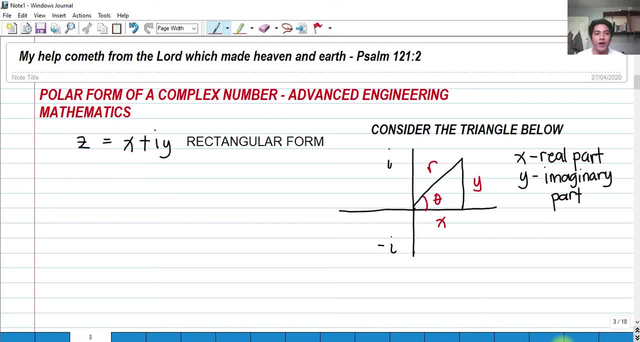 engineering mathematics. So let's get started. So the polar form of a complex number. So, if you're again to recall the complex number, it is actually represented by z and that is equal to x plus y, i, y, which means that the i here is the imaginary number which is equal to negative of square root. 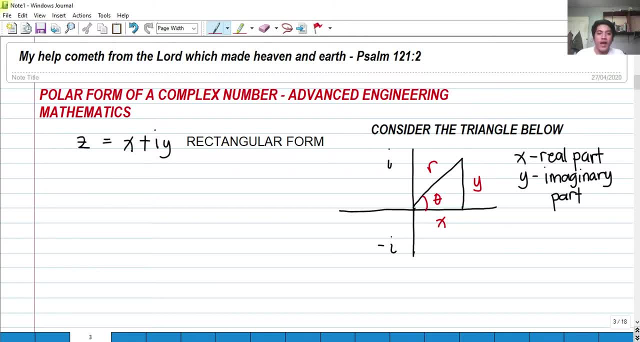 of one, and then we have x and y as real numbers, any real number. So we can represent complex number as this. So this is in rectangular form. So one plus i, two minus i, one half minus 0.5i. that is in rectangular form. So how do we get? 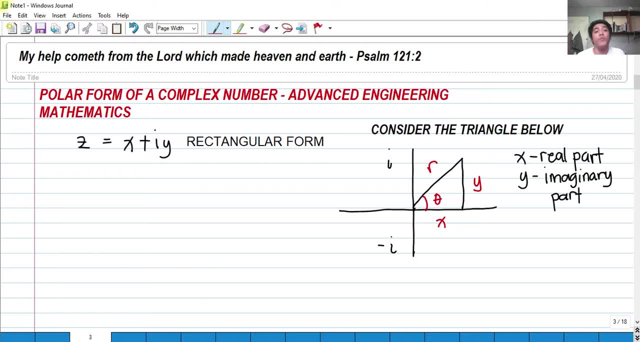 the polar form of a complex number from the rectangular form. So if we are going to consider this triangle below in an argand diagram, so we have the x-axis as the real part- okay, the real part here- for our complex number, and we have y as the imaginary part, okay, So 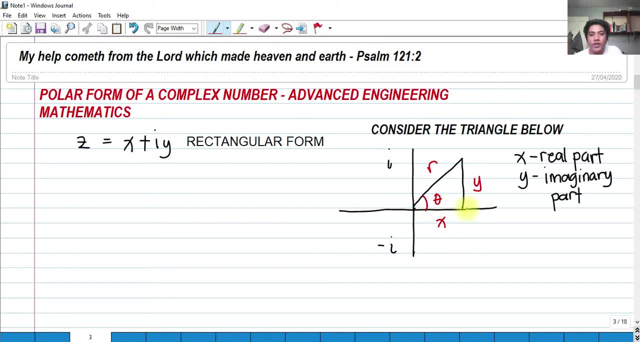 that we have positive real number here on the this one and then negative. we have positive i here and negative i here. So if we are going to draw, okay, let's say that we have a complex number in the form of x plus i- y. So if we are going to plot it in an argand diagram, so let's say that, 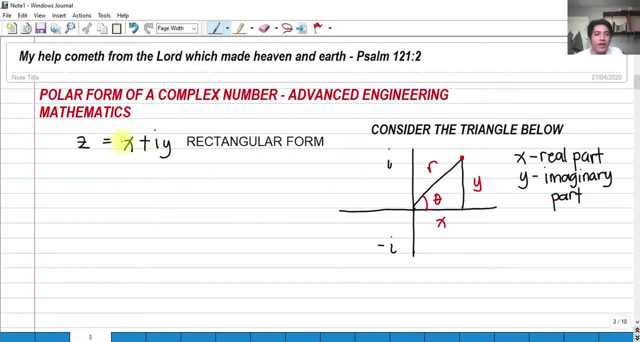 is this complex number represented by the coefficients of x and y. So what are we going to do Is that we have a certain value of x here, okay, the real number, and we have a certain value of y number here in the quadrant one, So it forms a triangle. We know that this is the x, this is the. 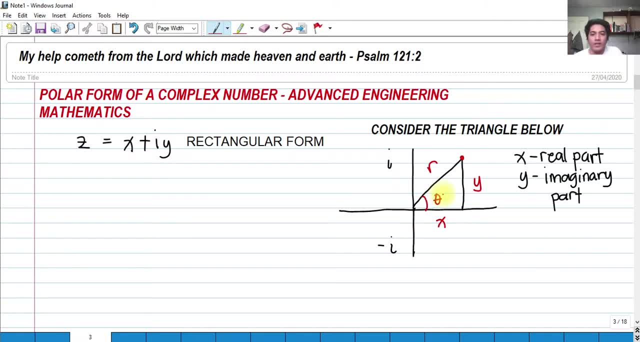 y, and what we actually want to get is the, what we call the r. okay, where r is r and theta represents the polar coordinates of the point x and y in the rectangular form, And r is what we call the. it is always a positive number. It is the length of the vector representing the. 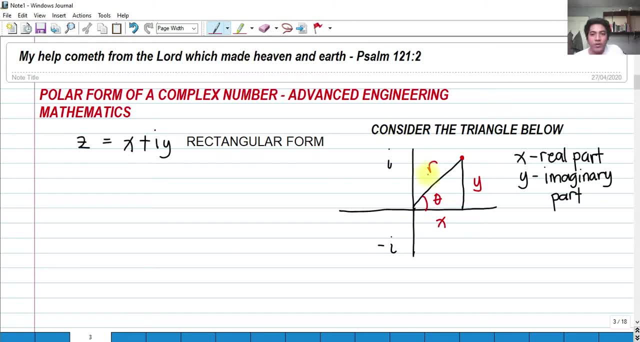 complex number say: okay, this r. So we know that by Pythagorean formula we can get r simply by the square root of x squared plus y squared, since this is a right triangle. So that's how we get r. the length of r, Again, r represents is a positive number, r It represents the length. 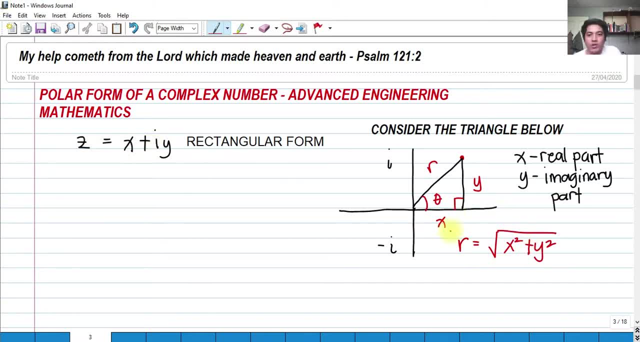 of the vector of the complex number say. So how do we get x and y? We can get x and y by having cosine, theta and sine theta functions. So for cosine we have adjacent over hypotenuse, that's x over r. And we have for sine theta, we have opposite over hypotenuse, So that is y over r. 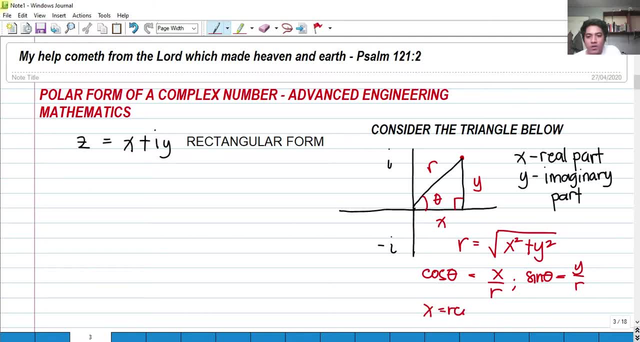 Getting x and y. so we have x equals to r cosine theta and our y would be r sine theta. okay, So polar form can be represented by the following: So, given these equations, so we know that z is equal to x plus iy. So what will happen here, since x now will? 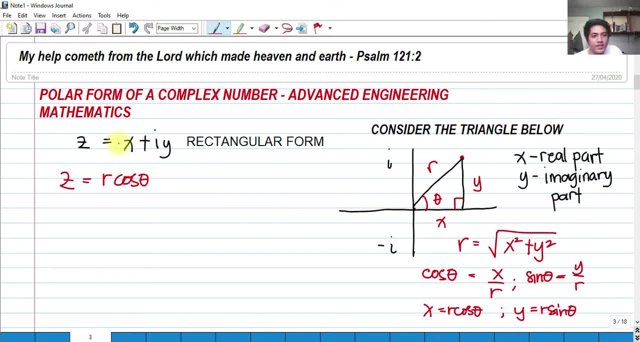 be equal to r cosine theta. we replace that this x plus we have, of course we have the i, that's the imaginary number, and the y, we have. r sine theta. Of course we can factor out r because it's common. So cosine theta plus i sine theta. 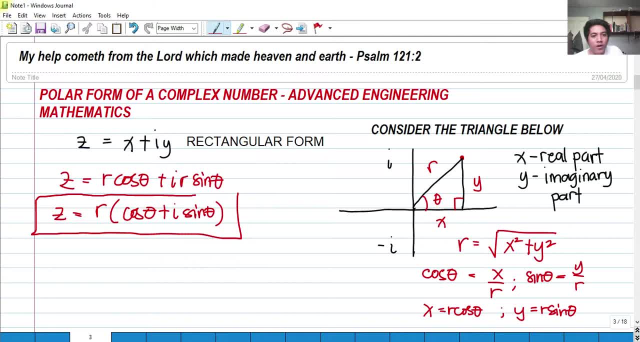 And this will be our polar form, okay, Our polar form of complex number. That is our polar form, okay. So how do we get this theta, Meaning this theta? we can get that theta by getting the tangent function, tangent theta that is opposite over adjacent. If we get 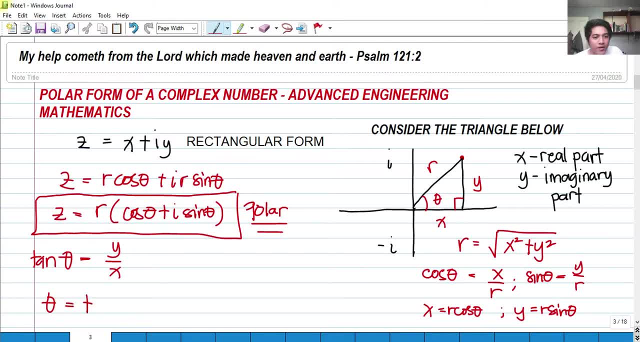 we wish to get the theta, that is, theta arctan. okay, y over x. So technically this would be our formula, but not all the time this will be used. okay, Because what if the x would become zero? okay, In such cases that the x would become zero meaning. 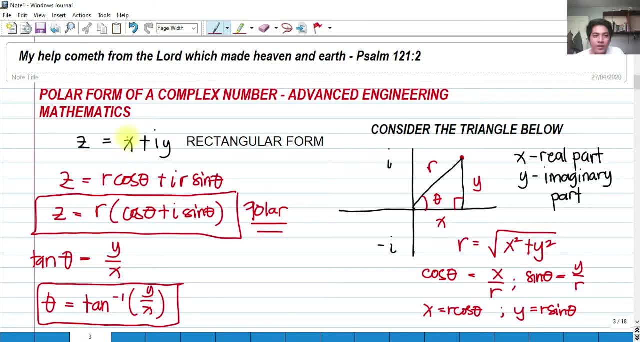 we don't have any real part. okay, Here the value of x is zero, so this would be undefined. So that only means that the angle is actually in the 90 degrees here. okay, Or pi over two, or negative pi over two. that would be our angle, In case that the y would be zero. 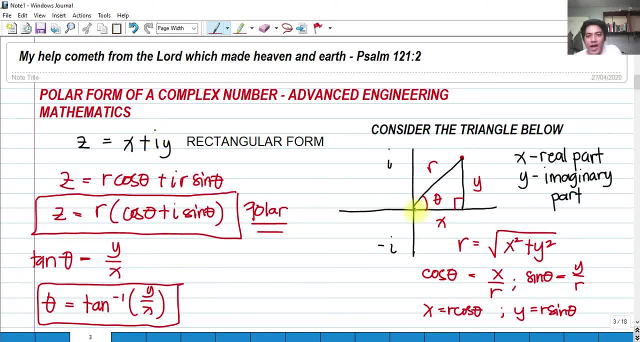 so arctan would be zero. okay, That's the first case. So the angle would be zero. or again, if the complex number is negative, okay in here. so what will happen? It would be lying on this part of our arctan diagram. okay, So, as we go on solving this formula or using this formula, 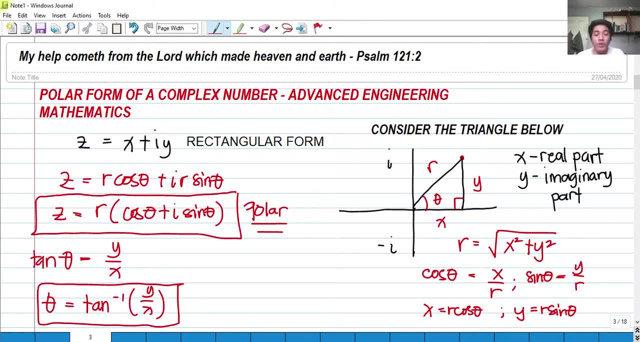 solving some rectangular form, converting it into polar. we will be tackling more about that, okay, So theta will be always it's best to express this in region. So it's best to. if you're going to use your calculator, it's always best if we are going to use that or make it in mode, region mode. okay, 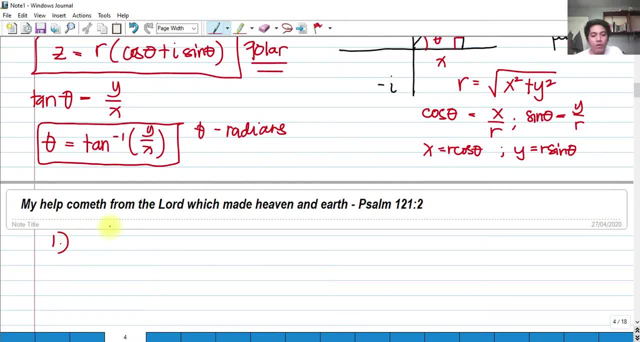 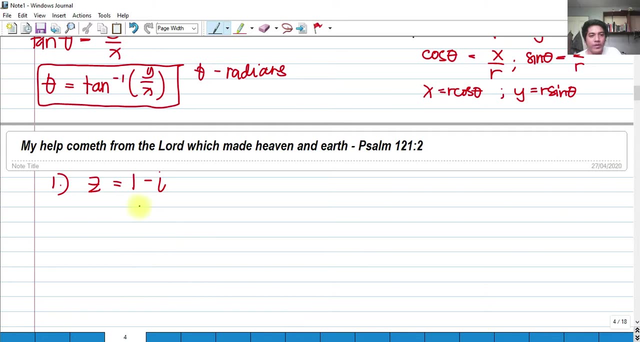 So let's try to solve some problems involving how are we going to convert complex numbers into its polar form? We know that this is in rectangular form, one minus i, So how do we, how do we convert this into polar form? So the solution for this is that we are going to convert or get. 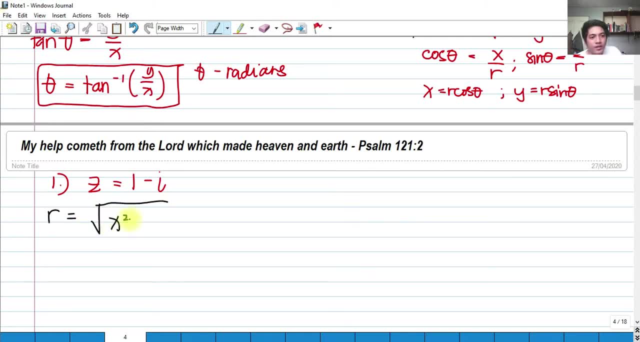 the r first. Again, the r is the square of some of the squares, of the square root, of the x squared plus y squared. In this case, our x here would be one squared, okay, The coefficient of x here. and then we have, plus the negative one squared, the coefficient of the imaginary part. 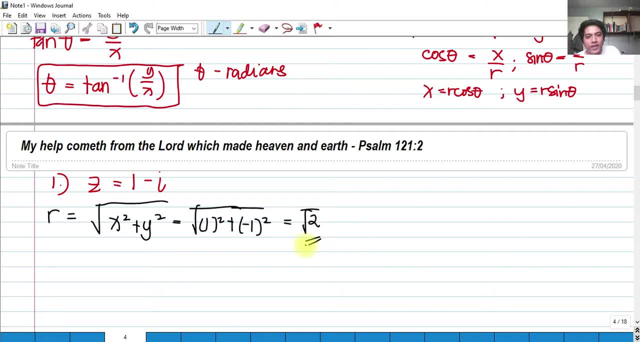 So we know that this should be the square root of two, and that is the length of our vector, the positive length of our vector r. We get the r. What do we need to get also is the theta, which is equal to arctan, of the y over x. We know that our y here is actually negative one over one. 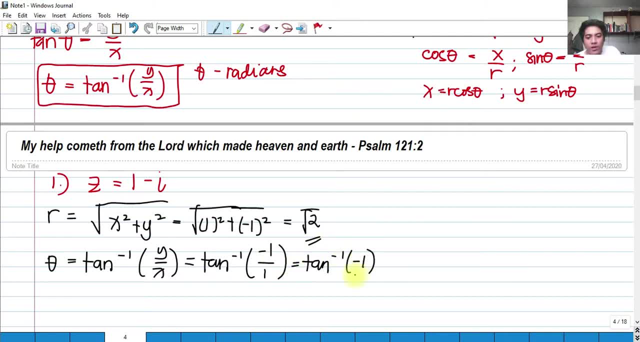 So that is simply the arctan of negative one, which is negative pi over four. So this is still correct, okay, Because we know that this rectangular coordinates lies in the fourth quadrant. This is in the quadrant four, Why? Because this is a positive value and this is a negative value. It lies on the fourth quadrant. 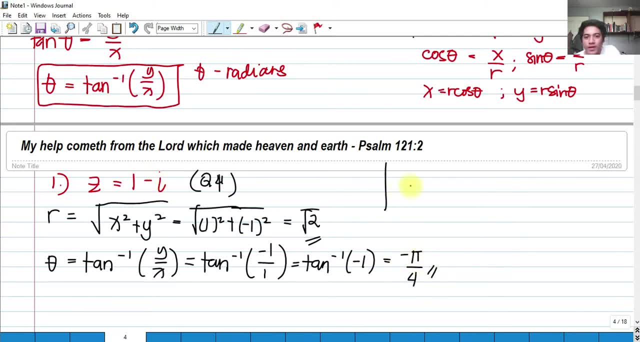 So this angle, though it may be negative, is still correct. So the negative only means that the angle is measured in the position okay, Measured from the positive x. positive x, The theta. I forgot to tell you that the theta is always measured from the positive x. That is our reference. okay, So our answer here. 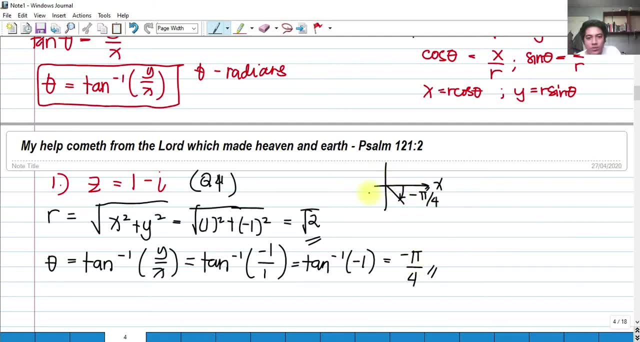 would be negative pi over four. or it can be also okay, three pi over four, okay, Three pi over four. or the supplement, I think okay. Okay, negative pi over four. I think we can also get the angle in the. 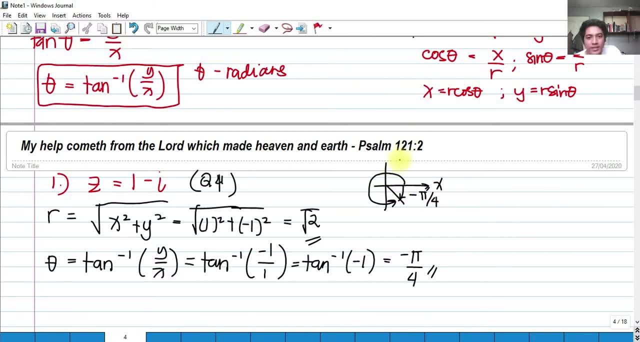 counterclockwise direction and that is seven pi over four, which of which is correct. But the calculator gives you negative pi over four, so we are okay with that, But we can also use seven pi over four as our answer. okay, So if we measure it counterclockwise, from the positive x. 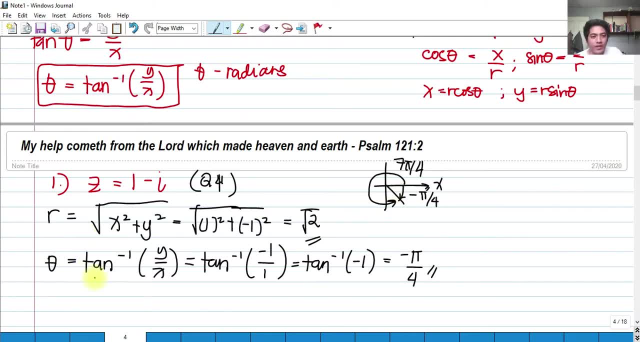 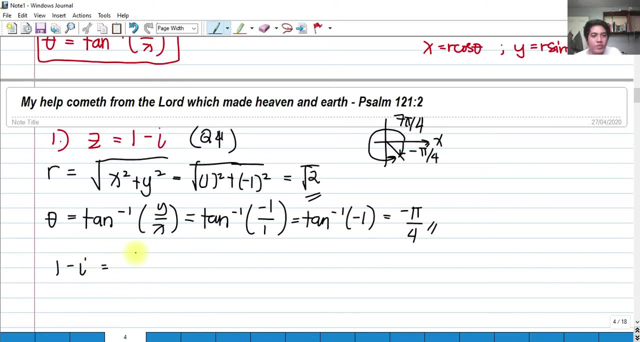 okay, So that is the answer for that. So if we are going to express this polar rectangular complex number into polar form, it should be this: The r, okay, The cosine of negative pi over four plus i sine of pi over four, and again. 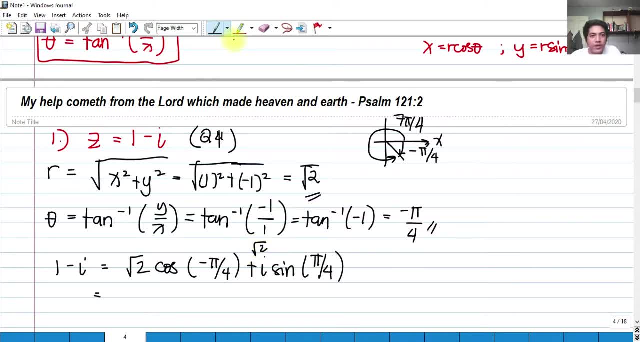 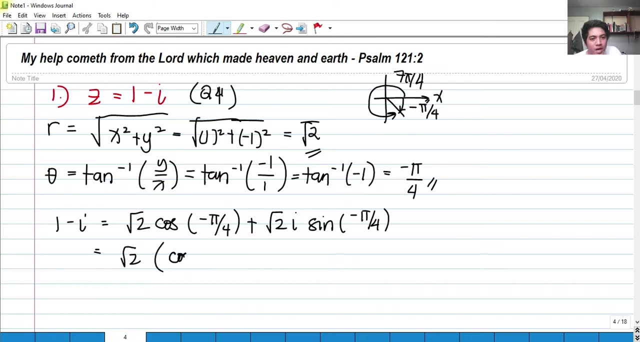 square root of 2 is common. i forgot square root of 2 here. let me just rewrite this: this should be r. also i sine of negative pi over 4. we can factor out square root of 2 because it's common. so we have cosine of negative pi over 4 plus i sine of negative pi over 4. so this is our. 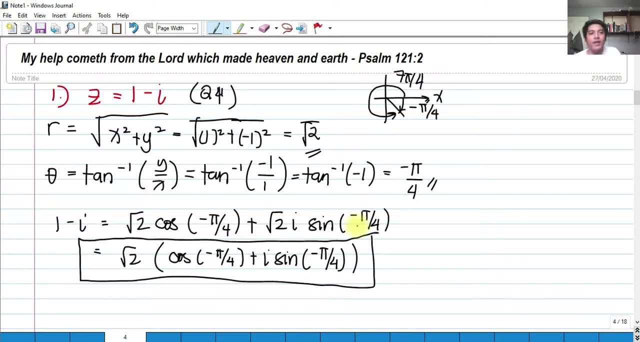 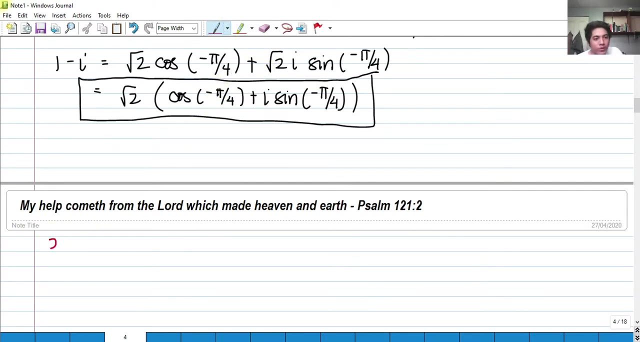 polar 4. for our answer in number one. again, if the complex number lies in the quadrant 4, okay, so we can. we can measure it, okay, clockwise or counterclockwise, from the positive x-axis. okay, for our second number, number two. so we have number two. we have to get the polar form of. 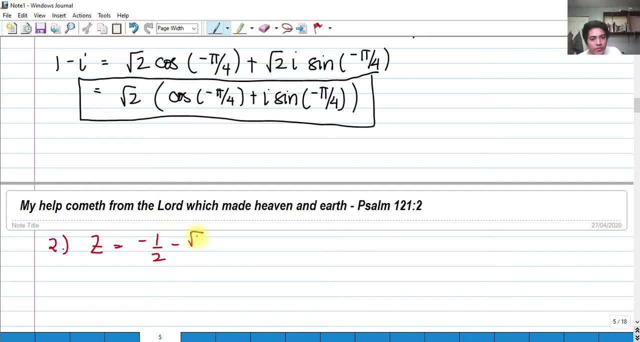 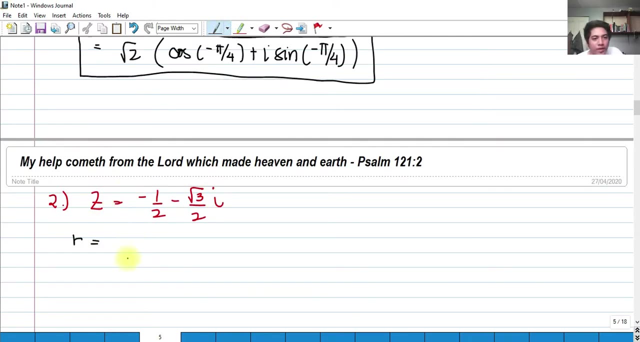 negative one half, okay, minus square root of three halves- i okay. square root of three halves- i okay. so again, this is pretty straightforward formula base. so we have to get the r, so we have negative one half squared plus a square root of three over two squared. and if 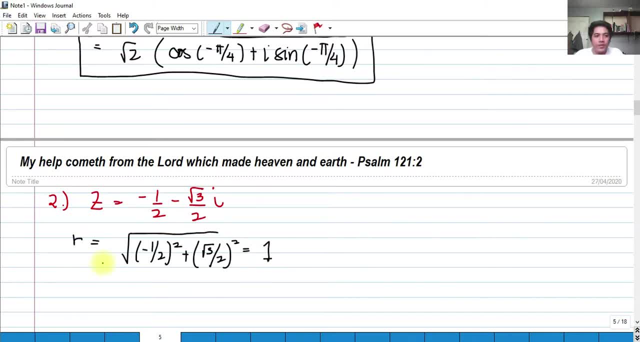 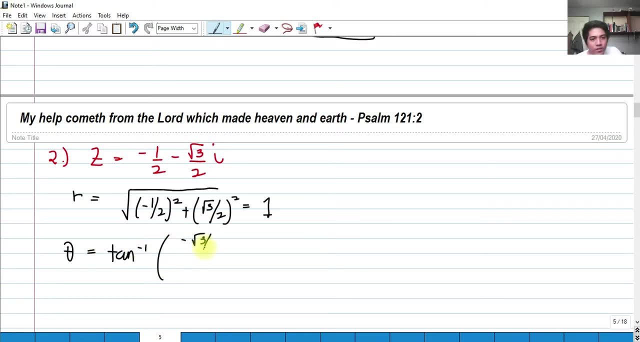 we are going to solve that. that's only equal to one. okay, then we get the theta of the arc tan of the negative square root of three over two over negative one half. so, as you can see, the twos will cancel. so we have, we are left with 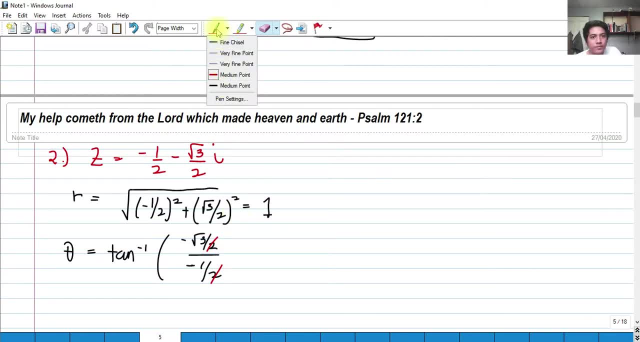 we are left with the arc tan of square root of three, because negative square root of three over negative one should be square root of three. okay, so that results for your calculator in pi over t. remember that your calculator always gives you the acute angle. okay, it's always an acute angle, but the theta here is: 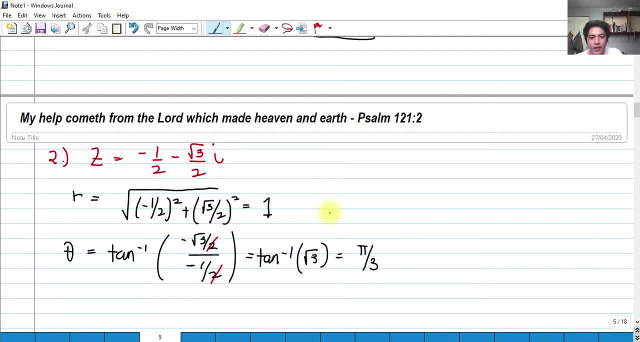 incorrect. okay, so the theta here is incorrect. we need to still identify first what quadrant does our complex number belong to? so we have a negative one, half squared over two squared over two, negative and negative. that's in quadrant three. so if, if it lies within quadrant three, upon getting 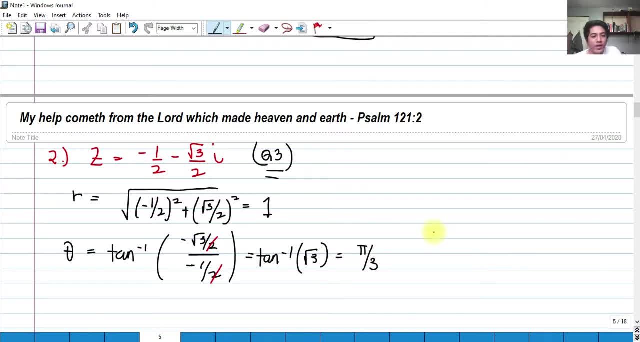 the theta from our calculator. okay, we need. so we need to add pi or subtract pi from this because, as we can see, this is our pi over three, our pi over three, whereas if we are going to analyze this complex number is in here, okay, so what are we going to do is simply, uh, we need to add it to pi, okay, or subtract it to pi. 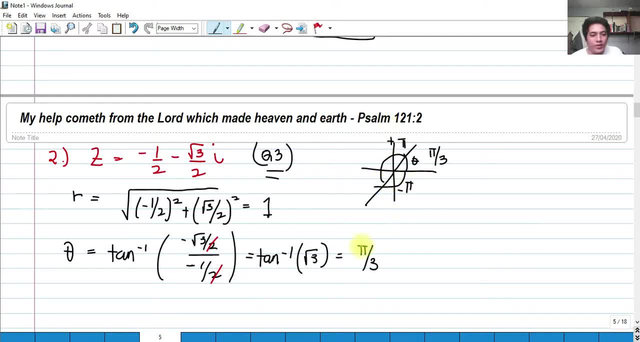 okay, add to pi or subtract to pi, doesn't matter, so we do here. it's more convenient to add pi. okay, it's, it's your, it's your call. okay, so if you subtract pi, this would be the angle. okay, okay, so the answer here will be four pi. 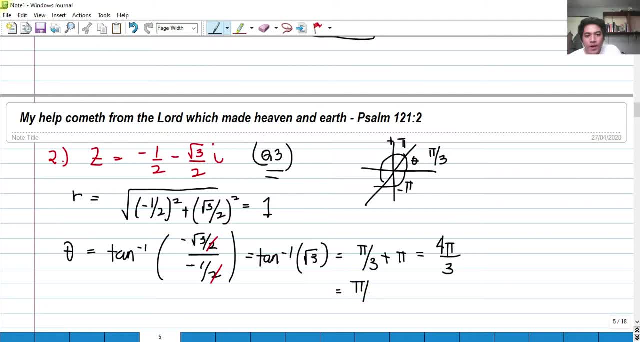 over three, or if you did pi over three minus pi, that is still the same. okay, as you will be in this coordinate or in this uh uh quadrant, okay. so what will happen if you use uh minus instead of plus pi? so you will be leading to negative two, pi over three, which is the same. 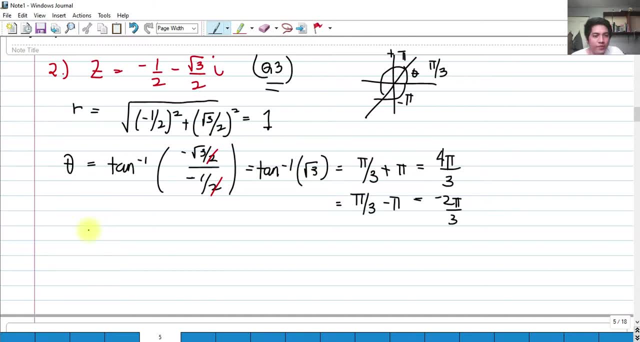 okay, so the polar form of this. you can choose one. so we have so negative one half minus square root of three over two, i is now equal to r, which is one cosine of theta, so cosine of four pi over three. plus i sine of theta, that's four pi over three. 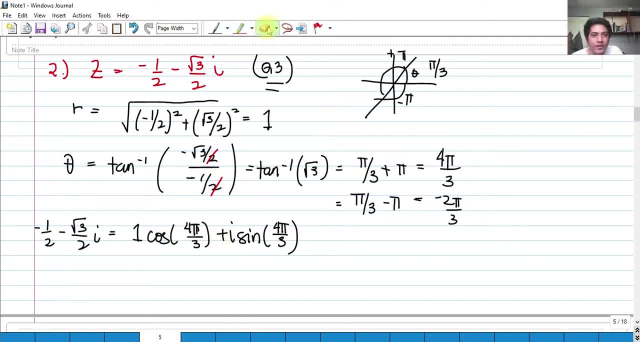 oops, we also have one here. okay so, but it doesn't matter. okay so that i'll delete the one here, because it's understood or it can be. it can be cosine of negative two pi over three plus i, sine of negative two pi over three, so 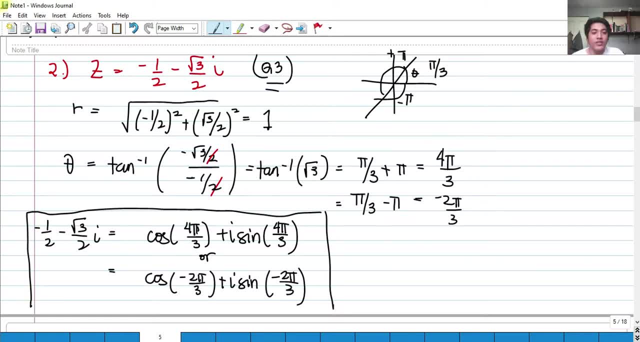 okay, that is actually our answer for number two. so, for for me, i always use if, if the, if the complex number is located in quadrant three, i always use a minus pi, but it's still the same. so for the rest of our example, if, if the complex number is located in quadrant three, i'm going to 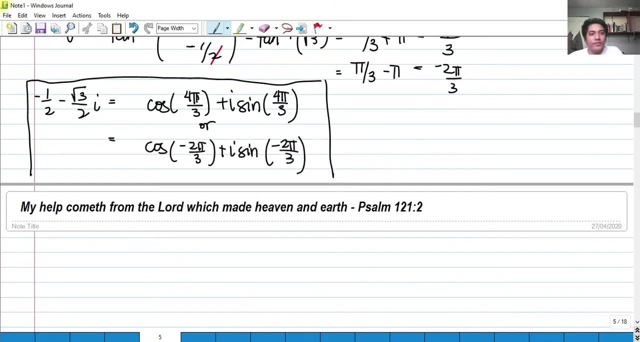 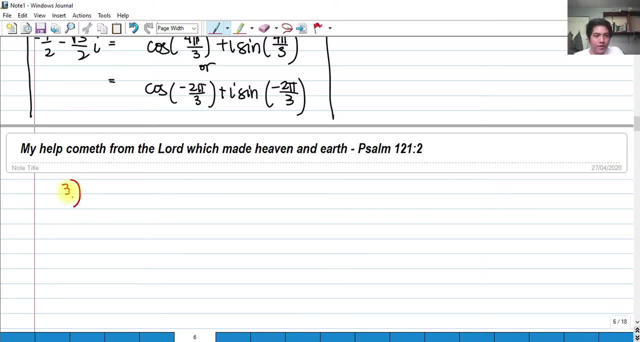 uh, subtract it from pi. okay, so let's uh try again another number. so for number three, okay, uh, we have the z is equals to negative one. okay, it's a complex number. it so happened that, uh, y has no value. so let's say, if we get the polar, 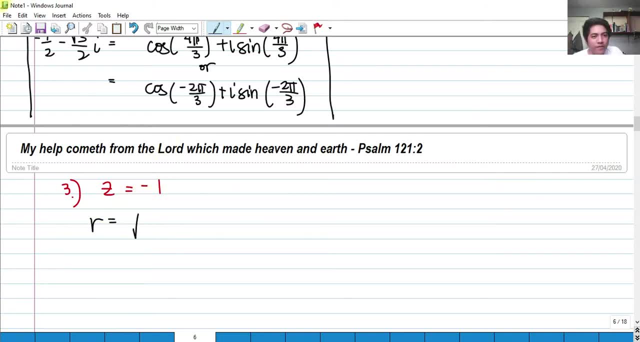 uh, form of this. so upon getting we have, we know that that is negative one squared plus zero, because it does not have any y value. so that's our r is still one. so our theta, that's ann of y over x, zero over one, that is art tan of zero, okay, which is actually zero. so 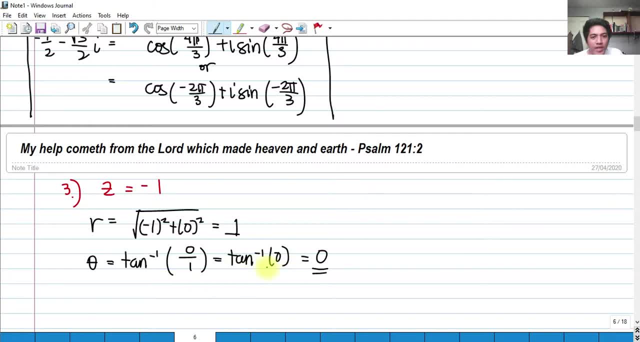 upon calculating with the calculator, it turns out that the angle is zero, but it is not if we are going to plot it. so this is our i, negative, i, this is our positive x-axis and this is negative one, and this negative one is located here. okay, and if we are going to measure the angle with respect to the positive, 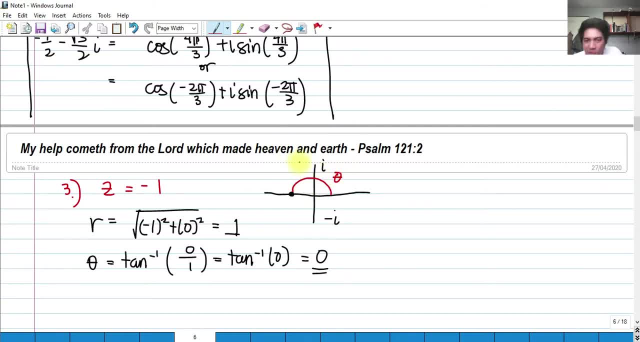 x-axis. that is not equal to zero, that is simply equal to pi. okay, that is simply equal to pi if measured. okay, our definition of theta is the angle from the positive x-axis. so this is our negative one. so our answer here should not be zero, but rather, okay, it is actually pi. okay, the angle. 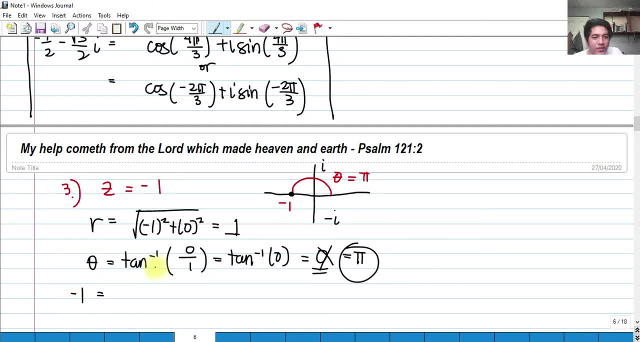 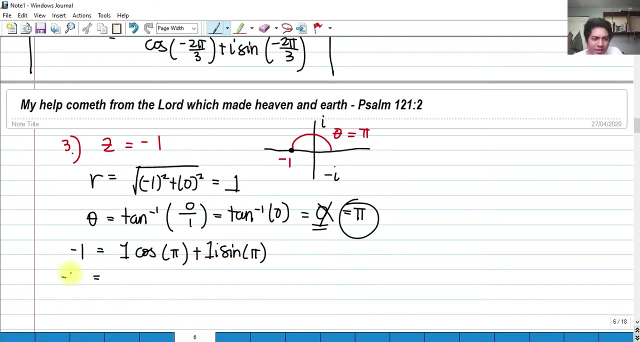 is actually pi. so in order for us to get the polar of this, that is, r cosine of pi plus i sine of pi, one i sine of pi, let me just rewrite this, even though we did not write one. it's okay, but still i'll write one here. okay? so we know that sine of pi is simply equal to zero, so we can leave it as. 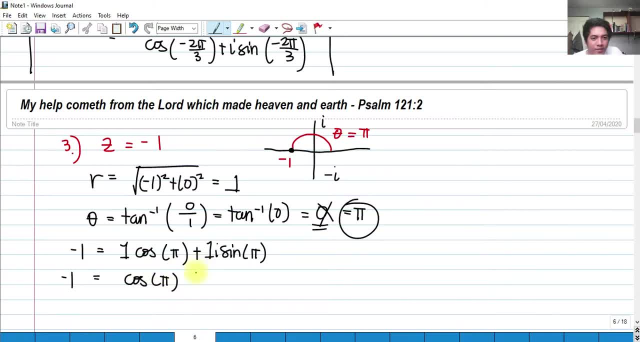 it is. so we have cosine of pi plus we have i sine pi. okay, if we are going to evaluate this, this is simply equal to zero. so we can leave it as it is. so we have cosine of pi plus we have i sine pi, negative one. so this is the polar form for our answer in number three. 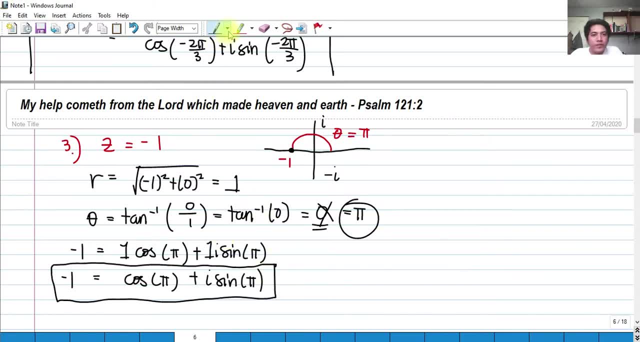 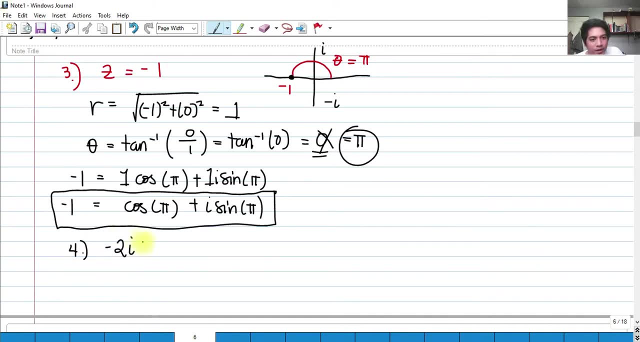 so how about for number four? let's try it: negative two, i, that's our complex number. so we get the r first. so our r is zero squared plus negative two squared, that is simply equal to two. okay, we get the angle, theta arc tan of y over x. our y is negative two, our x is zero. we cannot. 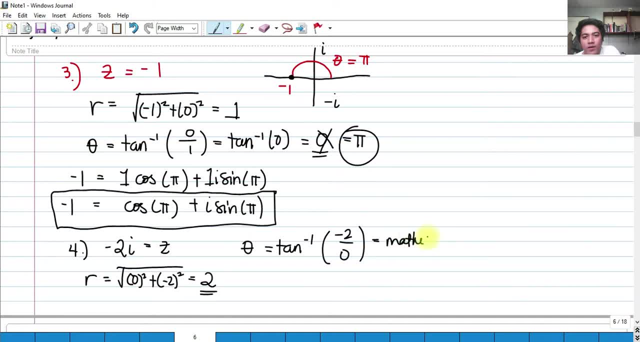 calculate, calculate this. this results to math error in your calculator because the denominator is zero. that that is math error in your calculator. but upon observation, by inspection, if you're going to uh, uh, graph, negative two y, this may be the negative two i. okay, negative two i. so it's located. okay, if we're going to measure the angle, 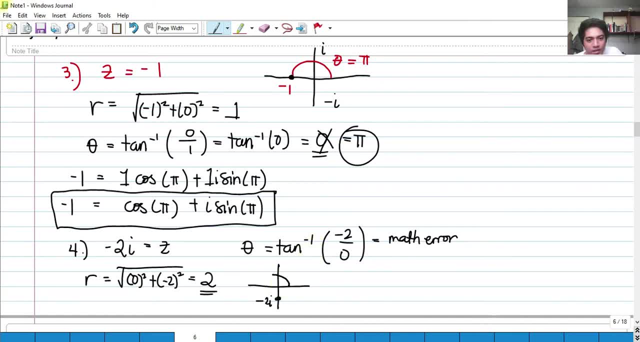 of this: okay, either from this, from counterclockwise or to clockwise. okay, we know that if we measure it from counterclockwise, okay, or clockwise here, from the clockwise here it is only equal to negative pi over two or negative 90 clockwise direction from the positive x axis. okay, so we can also measure. 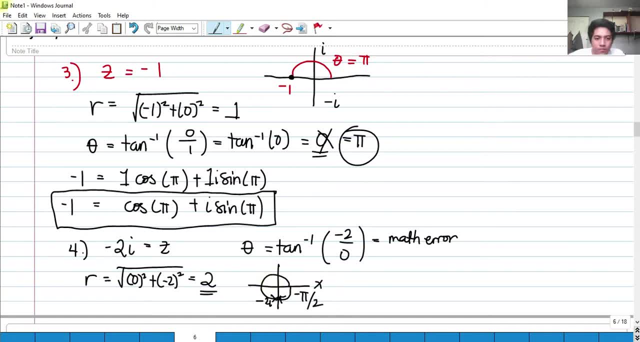 it here. okay, from the positive, and that would be three pi over two. but let's get this negative pi over two. so our answer in this question, negative two i is converted into polar form. that should be two cosine of negative pi over two plus two i sine of negative pi over two. so in other words, we can factor out two we have. 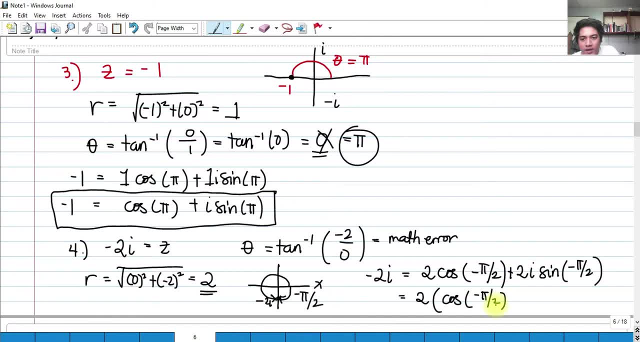 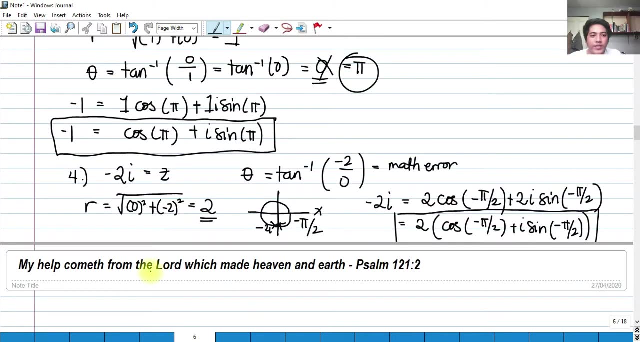 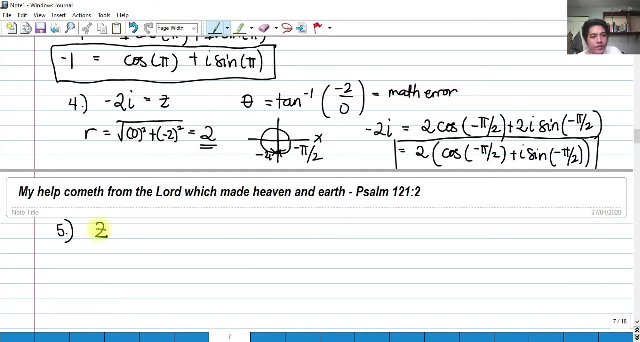 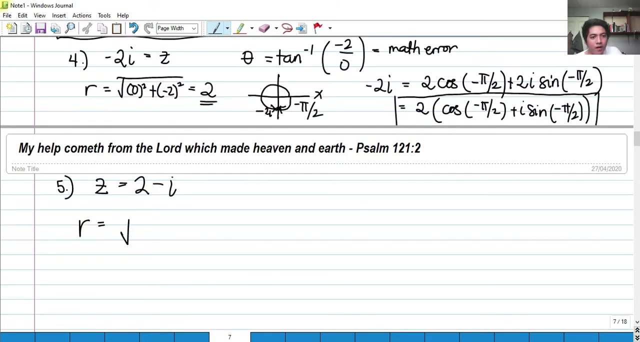 cosine two multiplied by cosine pi, two plus i, sine of negative pi over two. okay, this shall be our answer for this problem in converting this uh complex number into its four polar form to get the 네. so for number five we have, z is equal to two minus i. okay, so it's very simple. we get the. 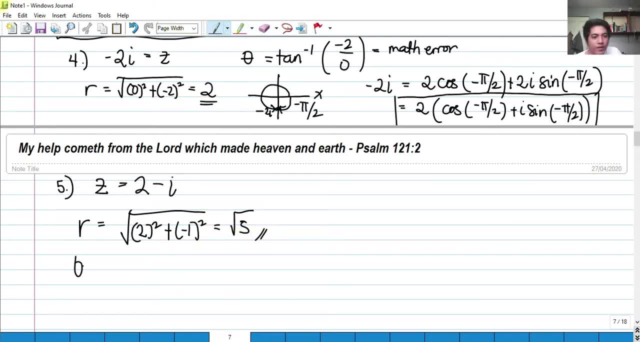 first, that's two squared plus negative one square. okay, that is square root of five. okay, so that is in our calculator. that's negative 0.464. okay, so it's correct. okay, take note that the negative here only means that it is measured, okay, in clockwise from the positive x clockwise direction. so 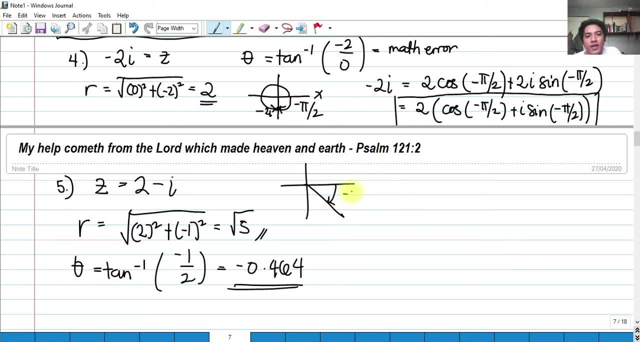 clockwise direction. okay, so that's negative 0.464. okay, not exactly in my drawing, but it's actually located here. that's our theta. our theta, okay. so if we are going to analyze, j lies in the quadrant four. okay, so we have the positive x, okay, and the negative y, so it. 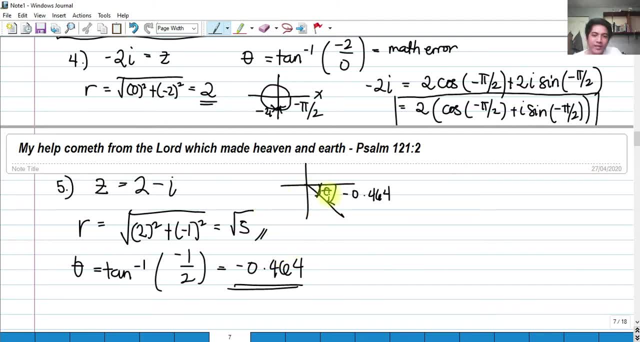 lies in the quadrant four. so we know that this is correct. okay, because we know that if the angle reaches here it should be negative pi over two and negative pi over two. you, if we evaluate that in decimal, that's negative 1.571 approximately in three decimal, so negative. 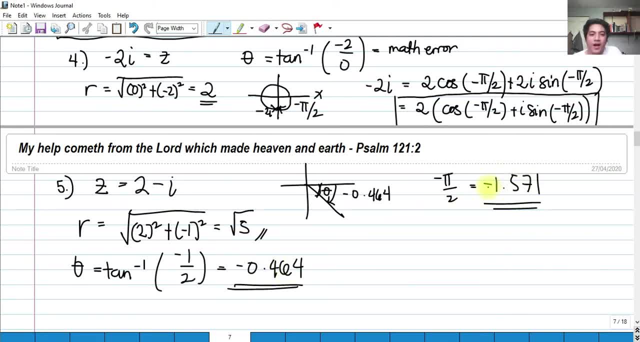 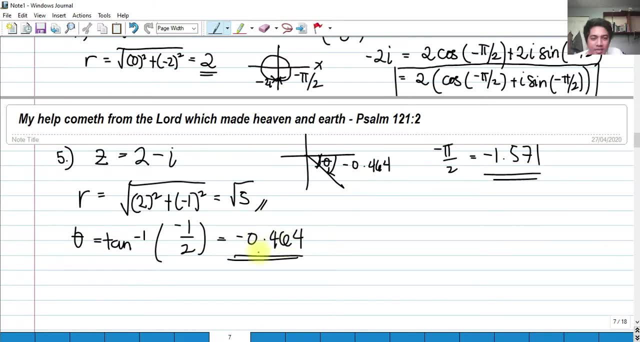 0.464 is less than this. i mean, uh, if we, if we neglect the negative number okay, which is still this is this should be correct, because it is less than this. okay than this, because it is this angle, okay, this angle is located at quadrant four. 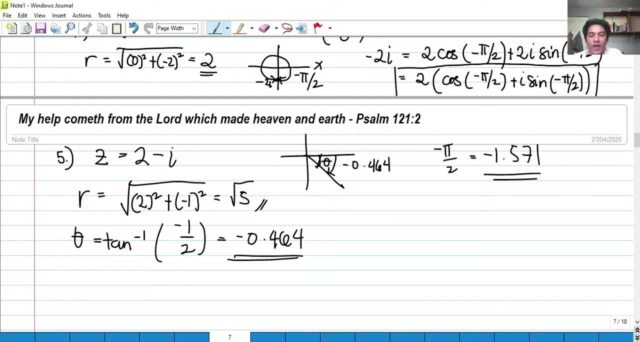 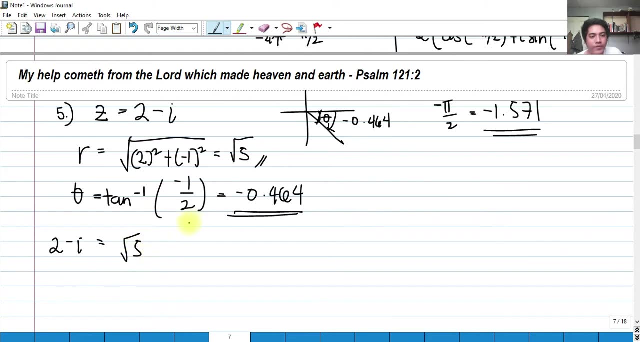 which makes our answer correct. so i hope you are able to get that. so our answer here for converting two minus i into its polar- uh, polar- coordinates, that would be square to five, okay, cosine of negative 0.464 plus i square to five. or square to five i, sine of negative 0.464. 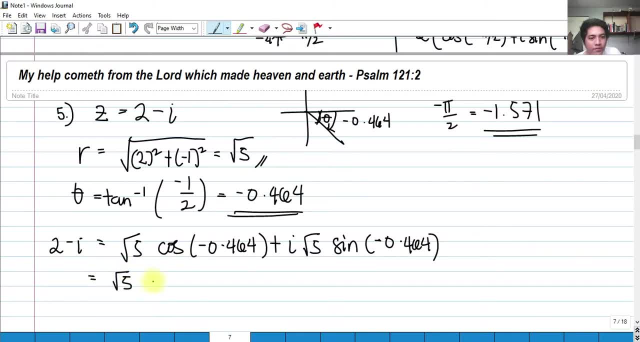 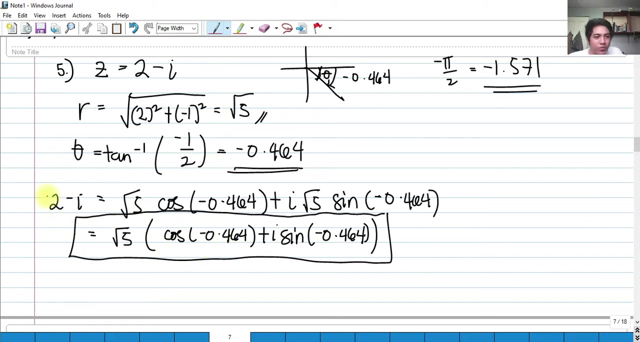 we can factor out square to five, so that we have cosine of negative 0.464 plus i, sine of negative 0.464, and here is our answer. okay, so let's try another problem. okay, so, by the way, if you evaluate this, this should be equal to two minus i. if that is not equal to two minus i, then our answer is not. 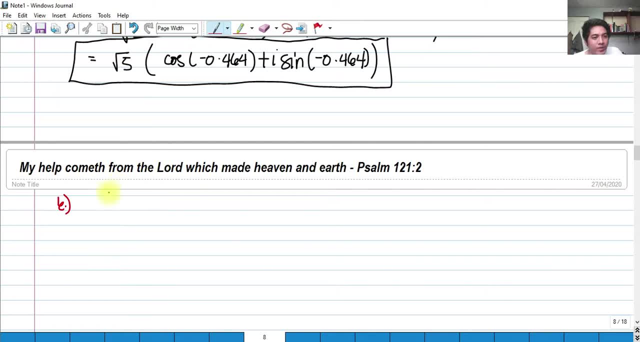 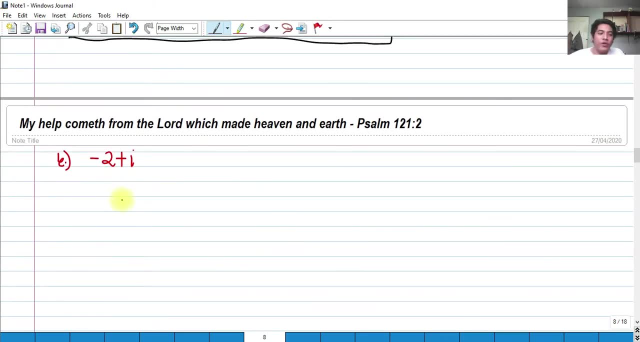 correct. okay, So 6 would be negative 2 plus i. That is our complex number. How do we convert this into polar form? So we have: r is equal to negative 2 squared plus 1 squared, So that is still equal to square root of 5.. 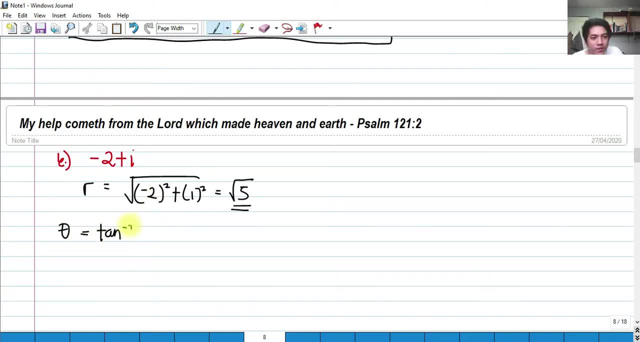 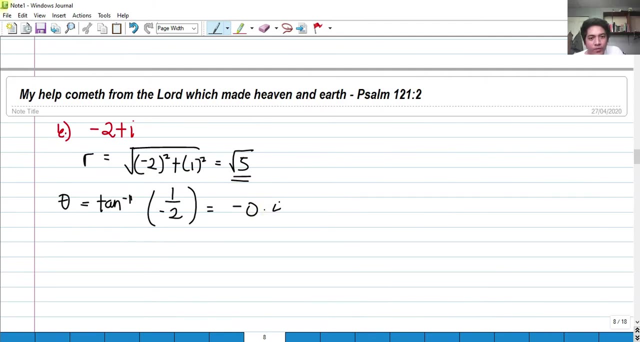 Our tangent or our theta would be r? tan of 1 over negative 2.. Which in turn, okay, which turns out. I mean that it is still equal to negative 0.464.. But if you are going to notice, this complex number is located in second quadrant, quadrant 2.. 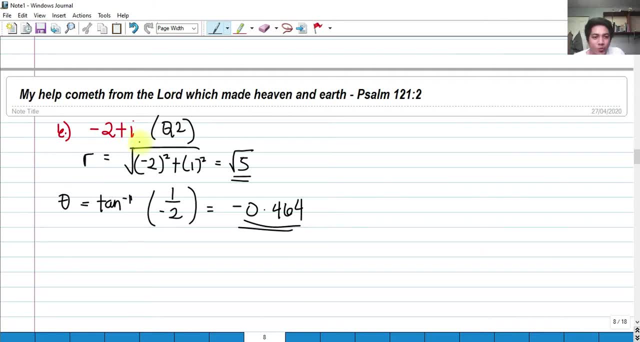 Negative x but positive y, that's in quadrant 2.. So what are we going to do is to simply add pi. Okay, plus a pi. So if we do that, okay, if it is in quadrant 2 plus pi, okay, just like what we did a while ago. 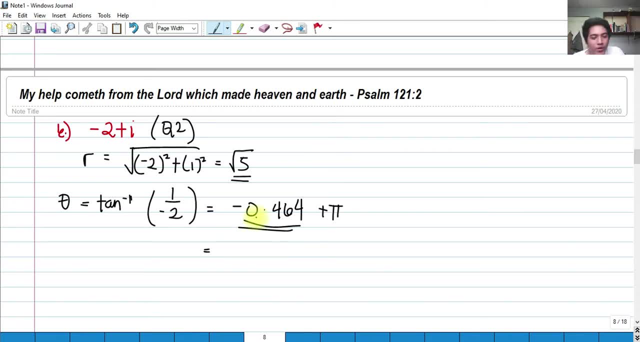 So we add pi. So that is 2.678 in 3D decimal, So 2.678.. That is our correct angle, because we know that this is measured. theta is measured from here. Okay, so we have to add pi. 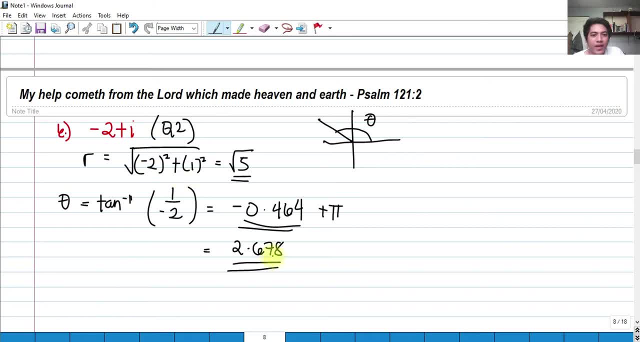 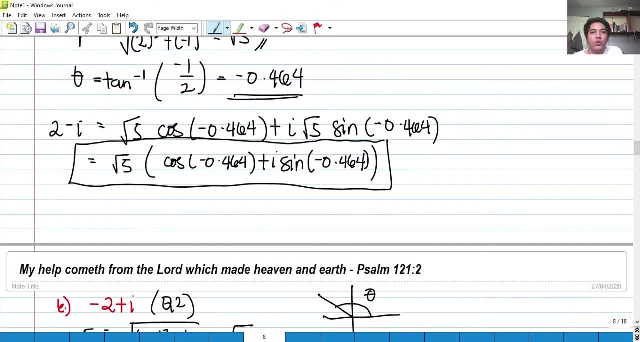 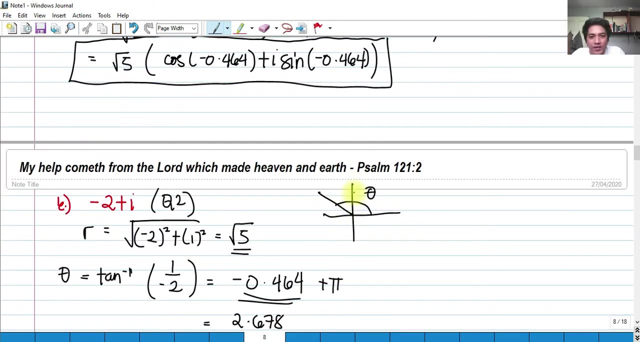 Okay, so okay, this should be our answer. It's greater than pi over 2, which is equal to. in this case, this should be positive, right? Because this one, if the angle is in this one, that's positive, 1.57.. 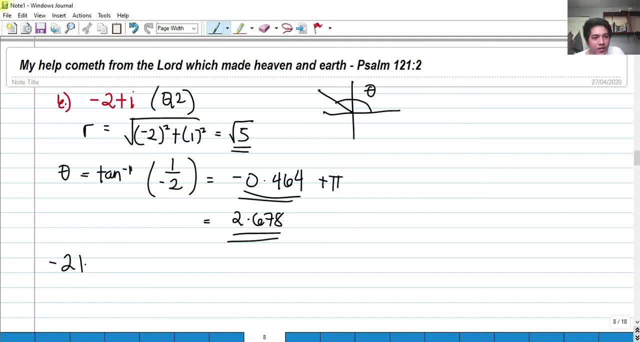 So we have this answer. So again, if we get the complex, I mean the polar form of this, it should be: square root of 5, cosine of 2.678 plus i, square root of 5 sine 2.678.. 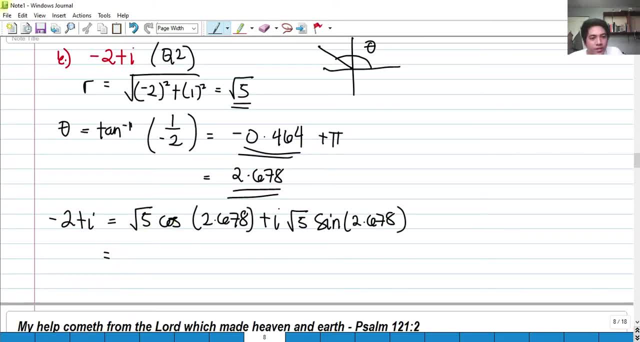 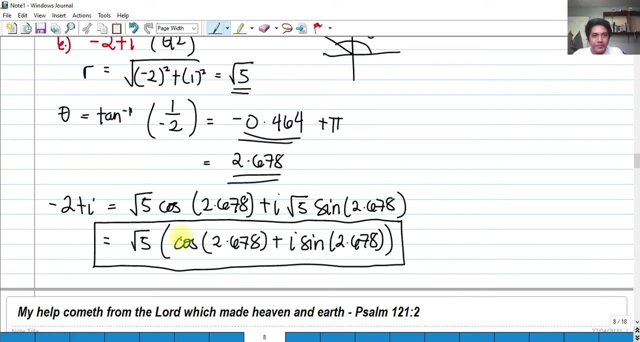 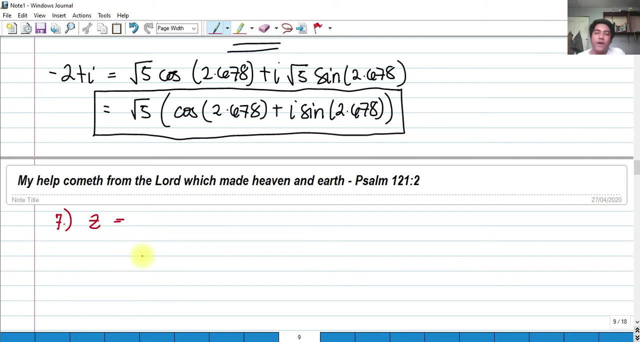 Since square root of 5 is common to them, that is, square root of 5, cosine of 2.678 plus i, sine of 2.678.. So this should be our answer for number 6.. Okay, so for number 7, it's pretty much the same. pretty much the same example. 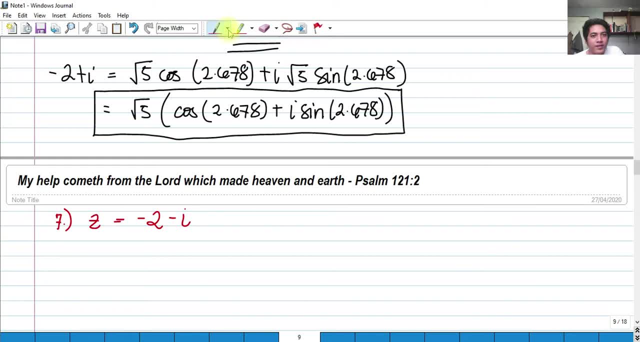 So we have negative 2 minus i. So how do we get that? So we have r. we have negative 2 squared plus negative 1 squared. Take the square root of that. That is still square root of 5.. And how about the theta? We have arc tan of negative 1 over negative 2.. 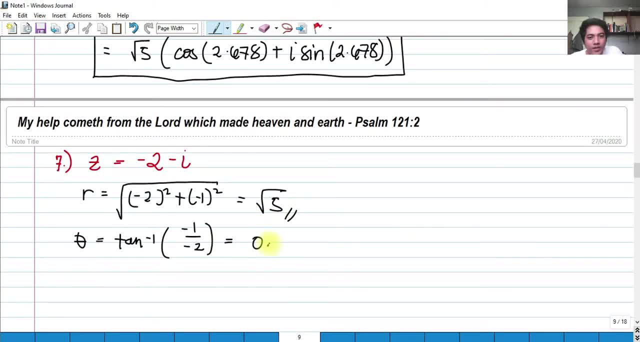 That's arc tan of 1 half, which it turns out to be 0.464, positive. But let me remind you that our complex number is located at quadrant 3.. So this angle is incorrect because 0.464 is in the first quadrant, which is here only. So we have to find the angle here. 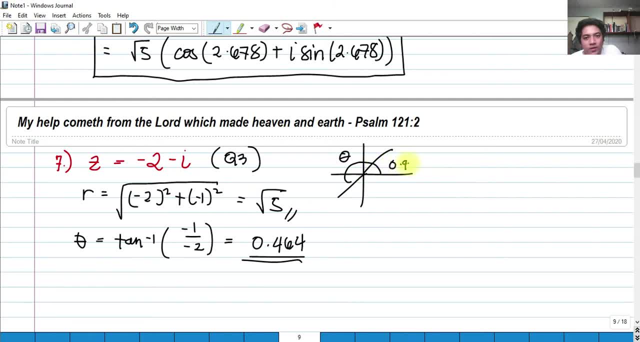 So if we get 0.464 here, okay, we can get, we can. let me just redraw this. This is our angle: 0.464 in terms of radians, but our angle supposed to be should be located here. Okay, So we have to add or to subtract pi here, Okay, Since this is in quadrant 3,. 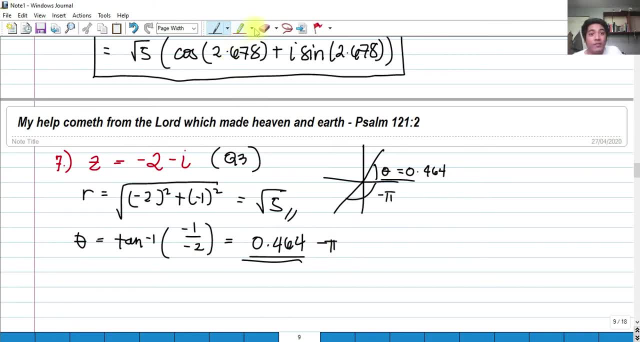 we have to subtract pi here. Okay, So that's what I'm telling you a while ago. Okay, That if it is quadrant 2 plus pi, if it is in quadrant 3 minus pi, So if we, if we subtract pi here, so we get. 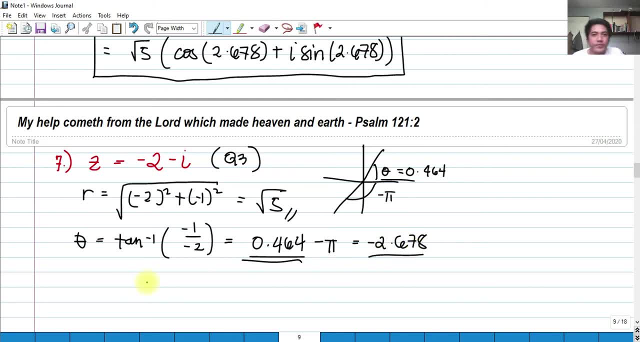 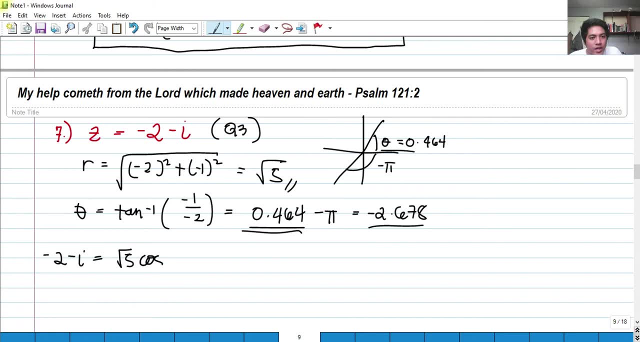 negative 2.678.. Such that if we are going to write the polar form of this, it should be: square root of 5, cosine of negative 2.678, plus square root of 5 i sine of negative 2.678.. Square root of 5 is common to them, So we have. 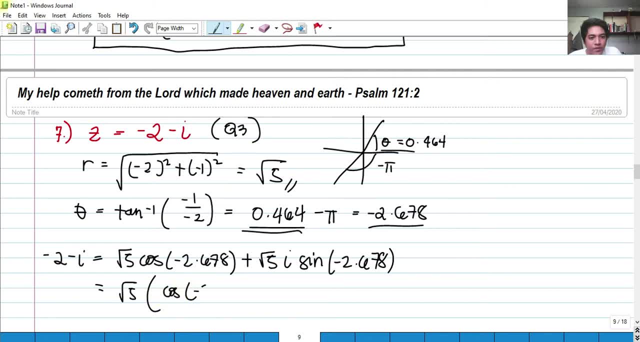 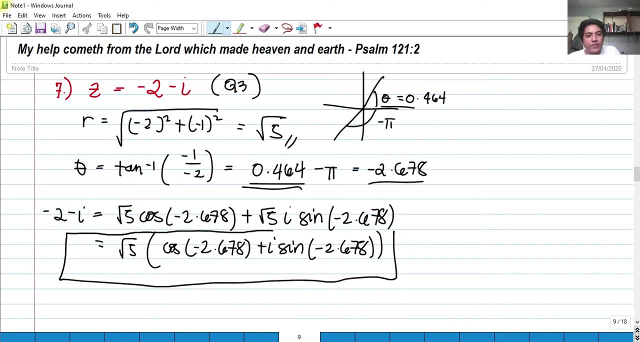 square root of 5, factor of square root of 5, cosine of negative 2.678 plus i, sine of negative 2.678.. So this should be our answer for this problem. So again, just take note if it is in quadrant 2 plus pi. 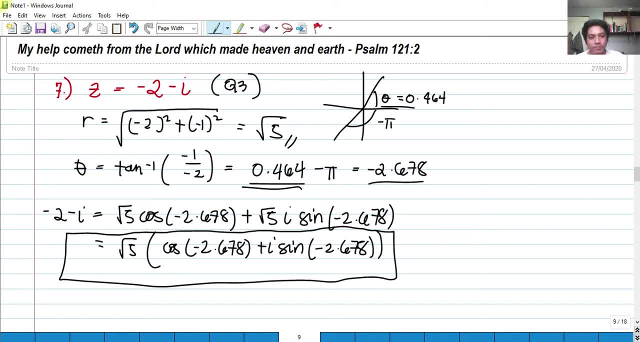 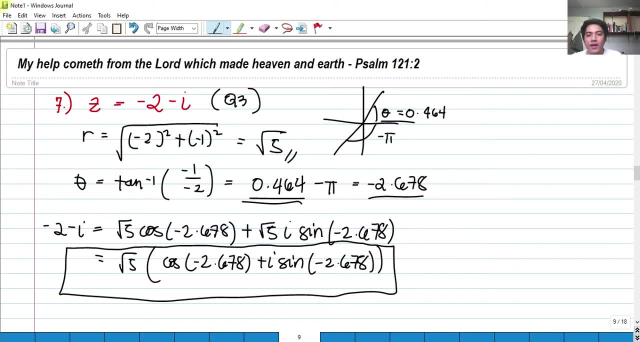 if it is in quadrant 3,, okay, minus pi. So for quadrant 4, it can be either plus or minus pi. If the angle that your calculator gave you is not correct, Okay, Or or or not correct in terms of. 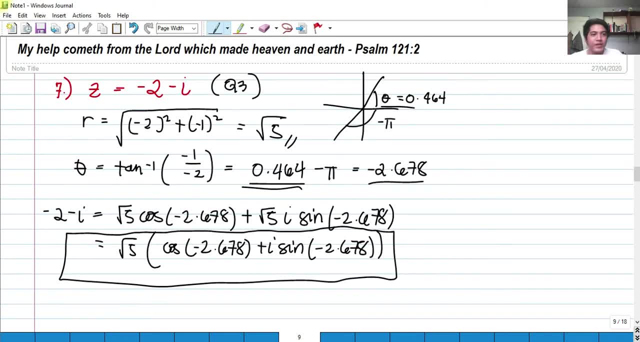 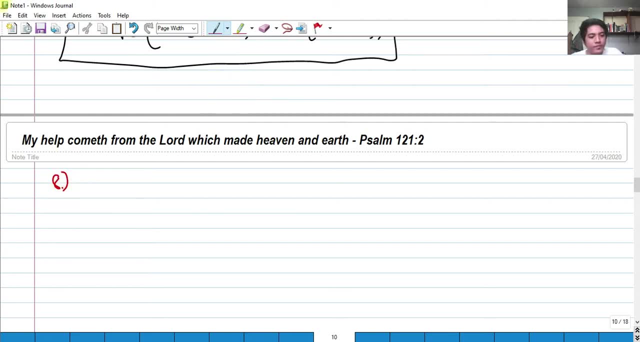 the quadrant. So if it is in quadrant 3, minus pi. So for quadrant 4, it can be either plus or minus pi Or the angle. Okay. So let's try the last example for number eight. So for number eight we have: 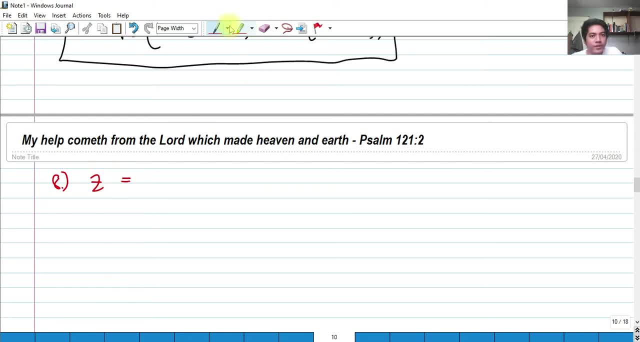 z is equal to: uh, I'm so sorry This is second to the last, Okay, So we have. we have: z is equals to equal to three, four negative one half i Okay, So get the polar form of that. So our. 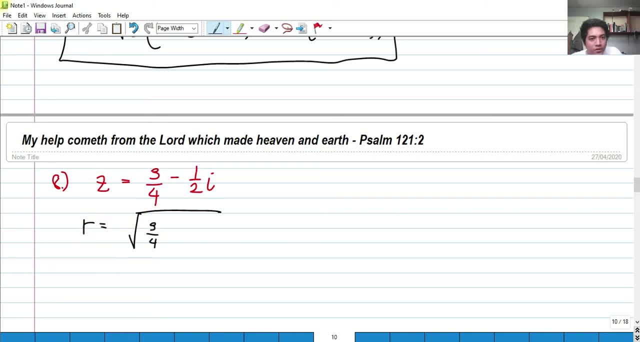 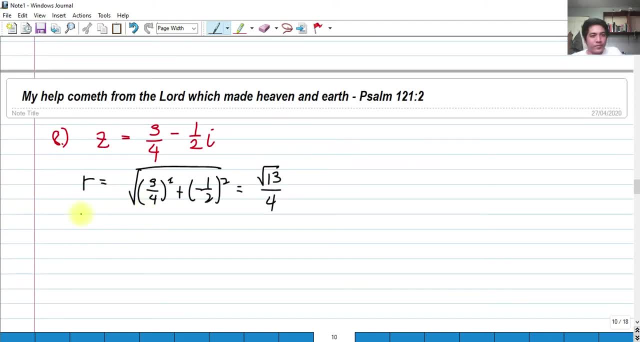 squared of 13 over four, The angle theta r tan of negative one half, y over x over three-fourths. So that would be in simple terms, We have four over two. So that is that would be negative two Thirds. The r tan of negative two-thirds is negative 0.588.. Make sure that you are in region. 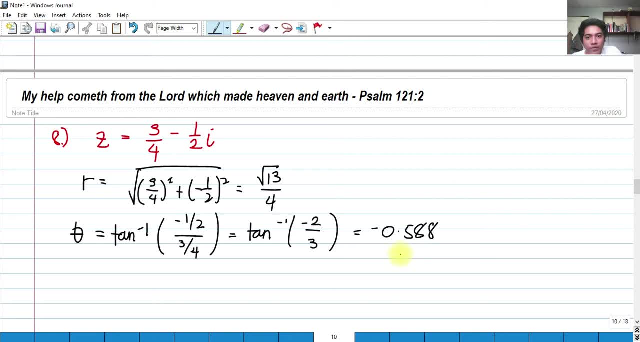 mode. Okay, So this negative 0.588 is correct because this is in quadrant four. Okay, This is correct because this is not greater than uh the pi over four, uh pi over two itself, or 90 degrees. One point or negative. 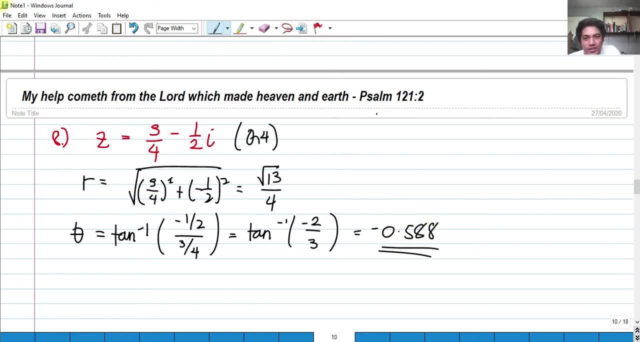 One point 57. So this is now correct. Okay, So this is now located, If we are going to measure it counter or clockwise, as negative 0.588, because if we extend the angle here 90 degrees, that is pi over two, which is negative 1.57.. So it is still correct. So the the answer that we have. 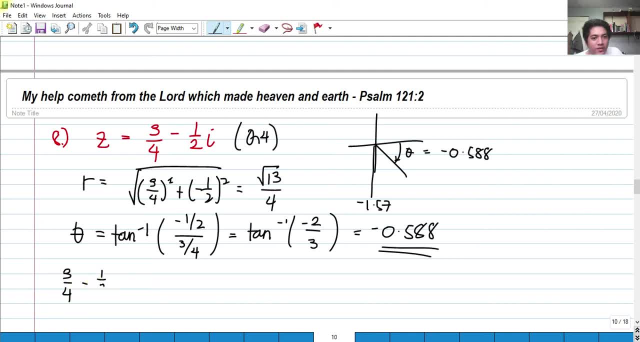 here is correct, So we can now therefore write it's complex Form. Our r here is square root of 13 over four. Let me just factor it out. Okay, So we have cosine of negative 0.588 plus we have, uh i, sine of negative 0.588.. So this is our answer for the. 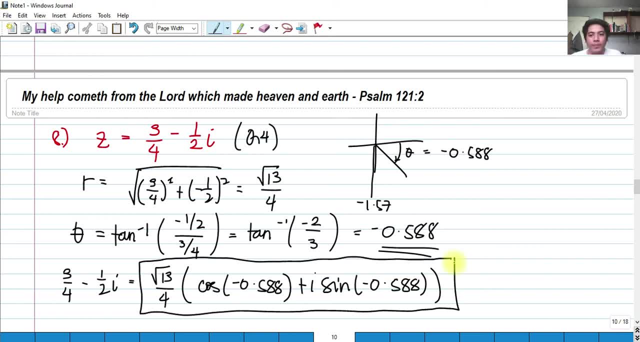 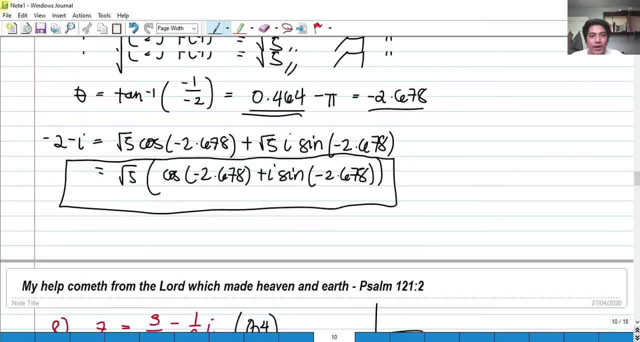 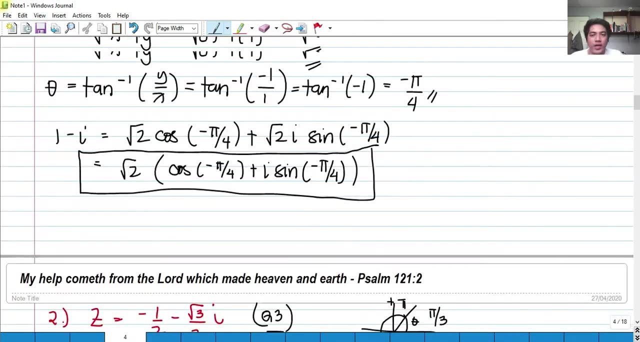 polar form for this problem And I hope you learned something for today's video In converting a simple- uh rectangular, uh uh complex number into polar form, And I hope to see you again on the next video. or, if you are new to my channel, please don't forget to subscribe and 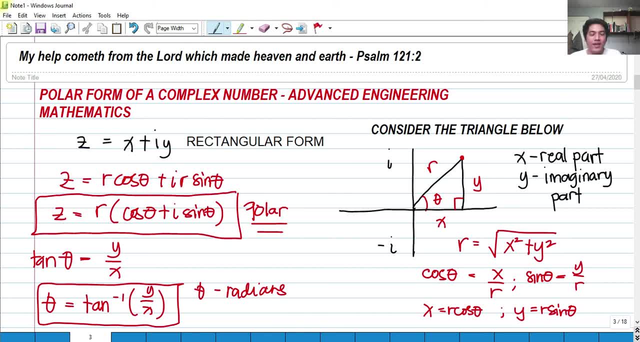 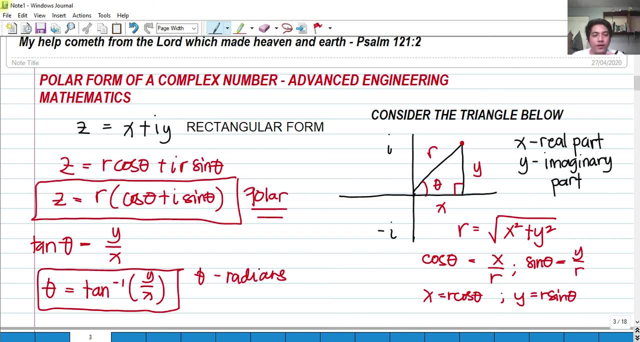 check out my playlist in advanced engineering mathematics. Okay And again okay. Simple reminder before we close. Okay, Uh, if the complex number is located in quadrant two, we we add pi. If it is located in quadrant three, we subtract pi. If it is in quadrant four, we can either add or 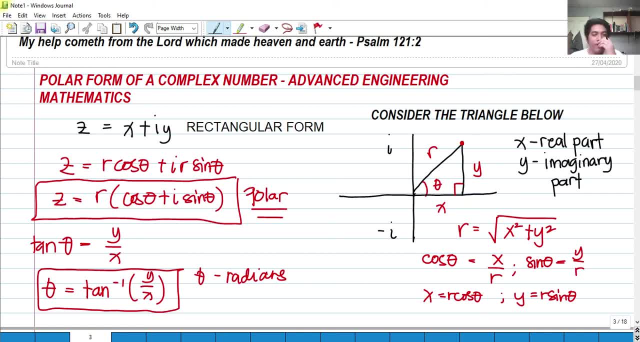 subtract. So thank you so much for listening. Uh, I hope you learned something today. Again, this is Engineer Abad. God bless you.